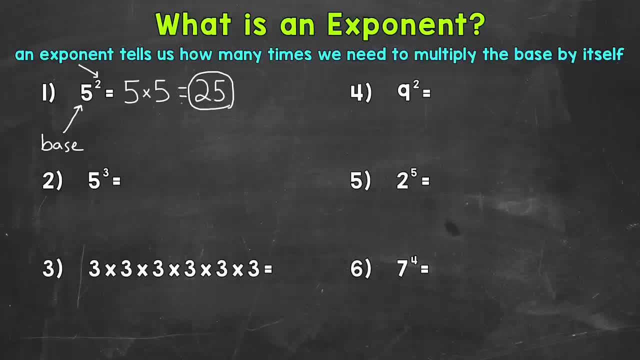 Another important aspect of exponents I want to cover is how to say them. For number 1, we can say 5 to the power of 2.. We can also say 5 to the second power, Or an exponent of 2 actually has a special name. 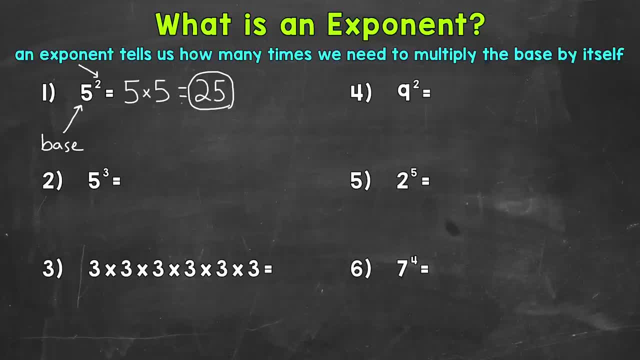 We can say 5 squared. Any number to the power of 2, we can say squared. Let's move on to number 2. Where we have 5 to the power of 3.. We can also say 5 to the third power. 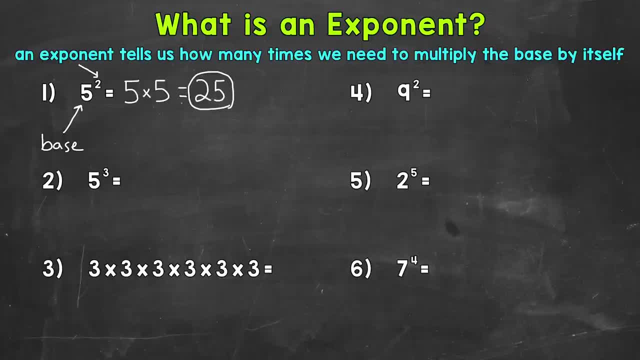 Or an exponent of 3 has a special name as well: Cubed. So we can say 5: cubed. Knowing squared and cubed is very important when it comes to exponents. For this one, we take our base of 5 and expand it out 3 times. 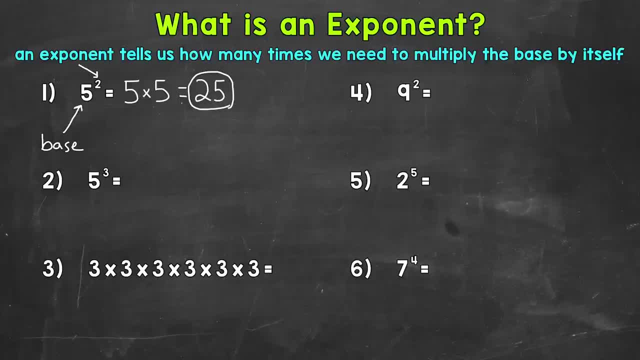 So 5 times 5, times 5.. 5 times 5, times 5.. Let's see what this equals. Well, 5 times 5,, that's 25.. And then we have one more 5.. 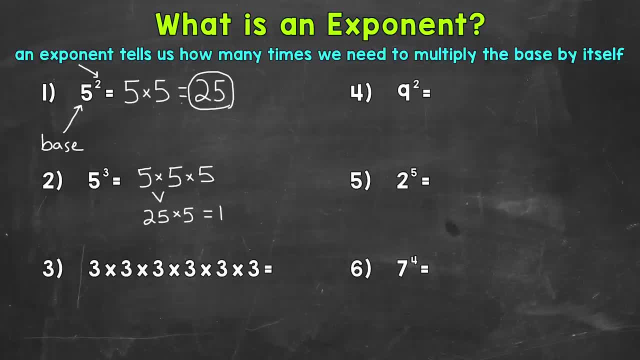 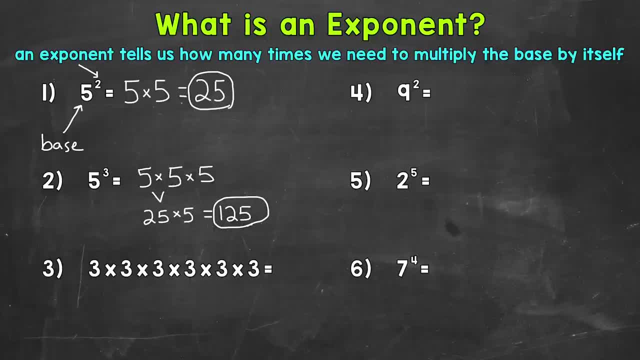 So it's currently in expanded form. Everything is expanded out. Let's write this in exponential form, So, as a base and an exponent, Our base is going to be the number that's expanded out, The number being multiplied by itself. 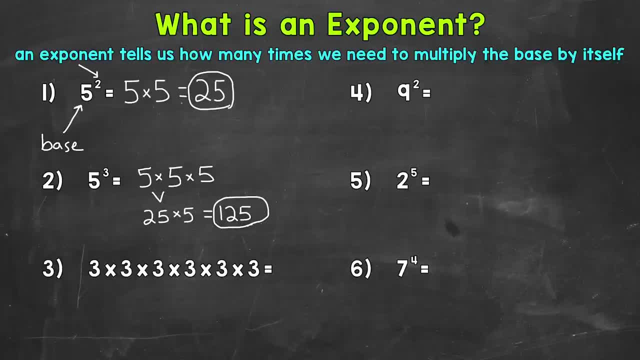 So in this case, Our base is 3.. Our exponent is going to be how many times that number is expanded out. How many times is that number being multiplied by itself? Well, 6.. So that's our exponent. So we have 3 to the power of 6.. 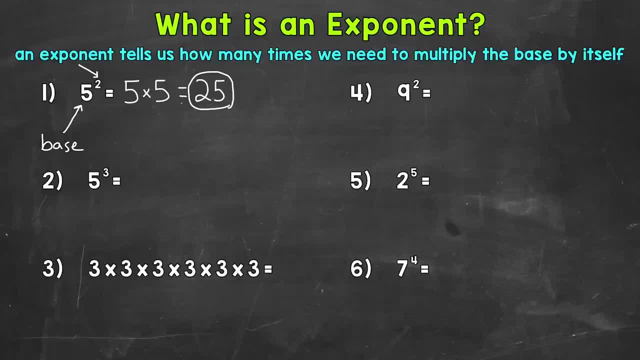 Another important aspect of exponents I want to cover is how to say them. For number 1, we can say 5 to the power of 2.. We can also say 5 to the second power, Or an exponent of 2 actually has a special name. 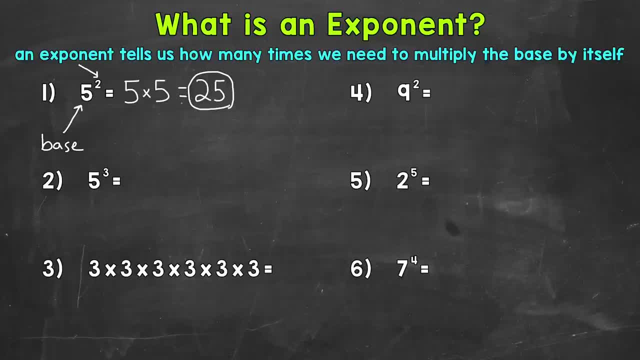 We can say 5 squared. Any number to the power of 2, we can say squared. Let's move on to number 2.. We have 5 to the power of 3.. We can also say 5 to the third power. 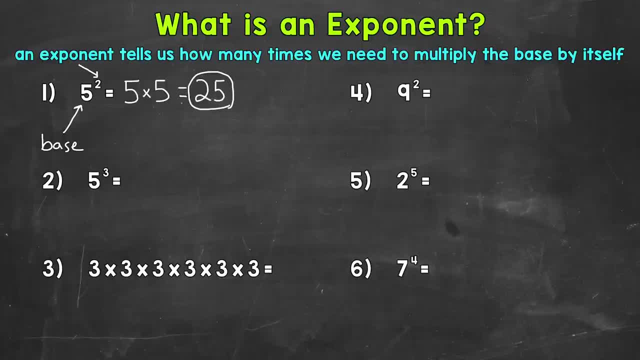 Or an exponent of 3 has a special name as well: cubed. So we can say 5: cubed. Knowing squared and cubed is very important when it comes to exponents. For this one, we take our base of 5 and expand it out 3 times. 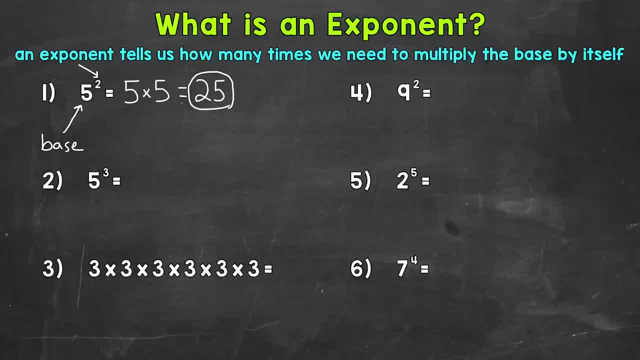 So 5. Times, 5. Times, 5.. 5. Times, 5. Times, 5.. Let's see what this equals. Well, 5 times 5,, that's 25.. And then we have one more 5.. 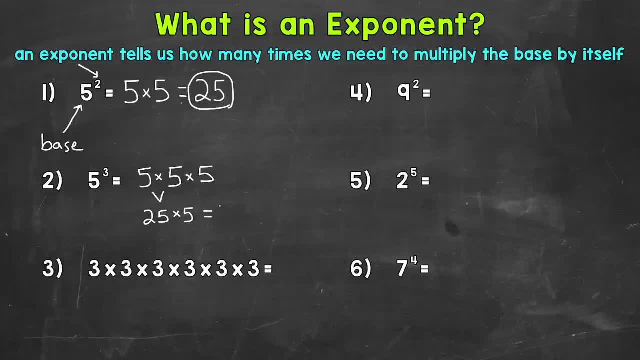 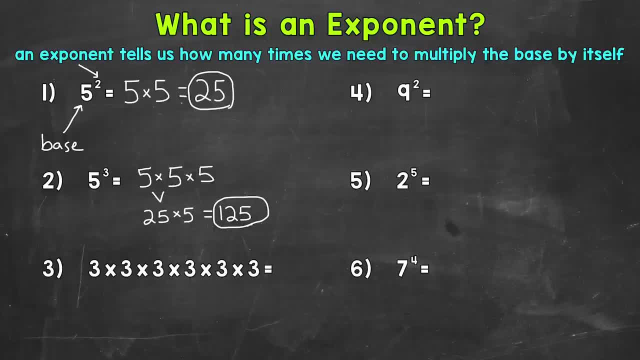 So it's currently in expanded form. Everything is expanded out. Let's write this in exponential form. So, as a base and an exponent, Our base is going to be the number that's expanded out, The number being multiplied by itself. So in this case, our base is 3.. 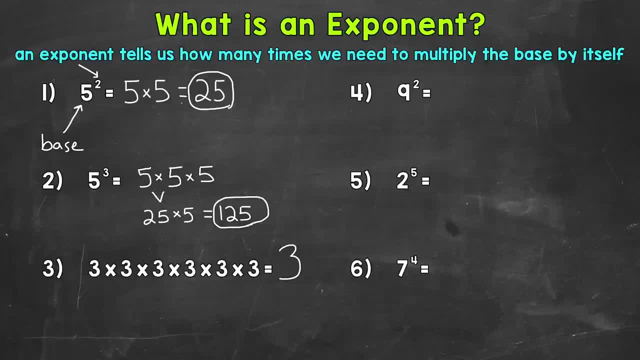 Our exponent is going to be how many times that number is expanded out. How many times is that number being multiplied by itself? Well, 6.. So that's our exponent. So we have 3 to the power of 6, or 3 to the 6th power. 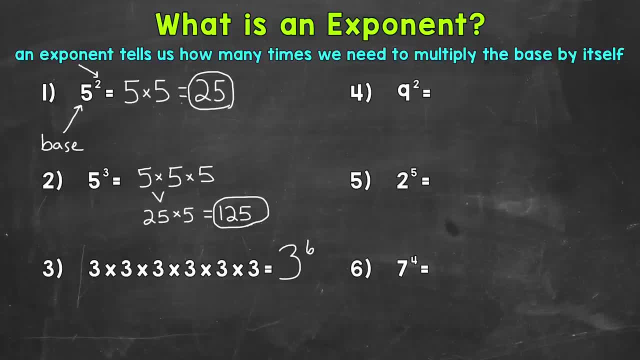 Or 3 to the 6th power. Let's see what this equals. Let's multiply everything here, And there are multiple ways we can Think through this and see what this equals. I'm going to pair up all of our 3's here. 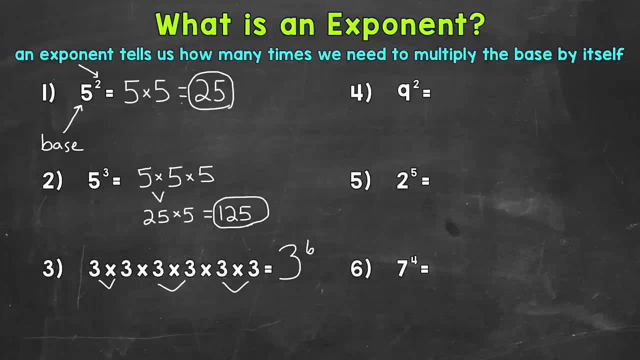 So we have 3 times 3,, 3 times 3, and 3 times 3.. We know that 3 times 3 is 9.. So I'm going to start breaking this down And let's multiply 9 times 9 times 9.. 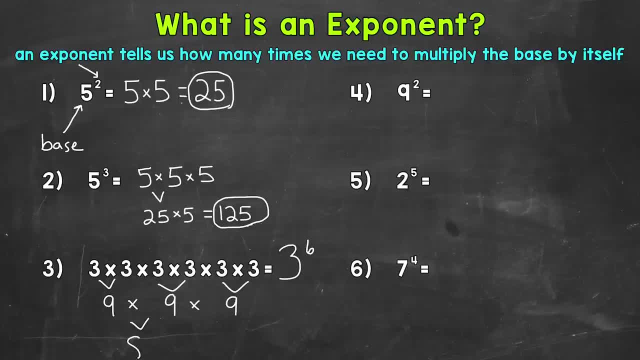 Well, 9 times 9.. That's 81.. And 81 times 9.. That's going to be 9 times 9.. That's going to give us a final answer of 729.. So 3 to the 6th power equals 729.. 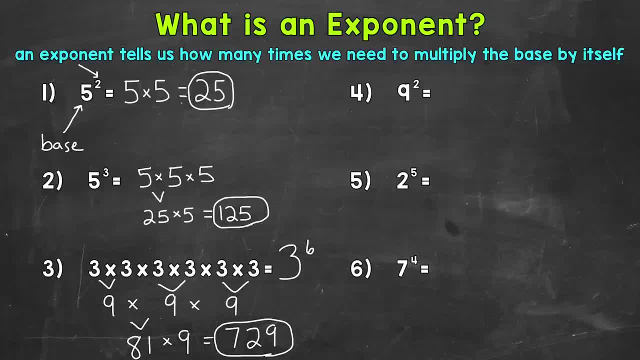 And, like I mentioned, there are different ways to think through that And different paths you can take in order to get to that 729.. For example, you can just start multiplying 3's as well. So 3 times 3 is 9.. 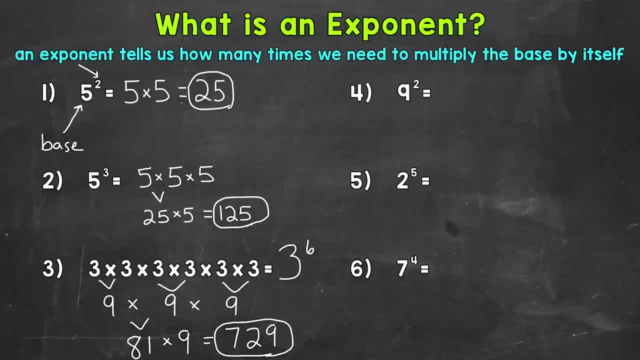 Then multiply that 9 by 3. And then that by 3. So on and so forth until you use all 6 3's. Let's move on to number 4, where we have 9 squared. So this means 9 times 9.. 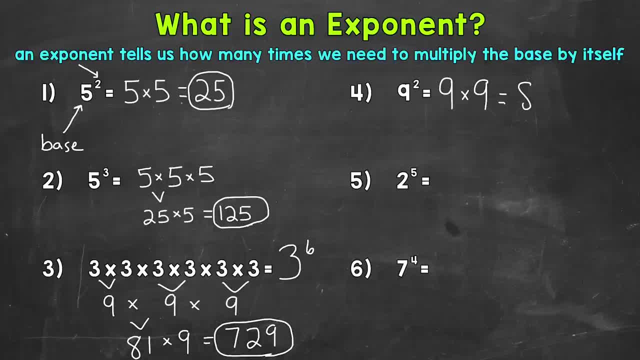 9 times 9 equals 81.. So 9 squared equals 81.. Let's move on to number 5, where we have 2 to the 5th power. So this is 2.. Times 2.. Times 2.. 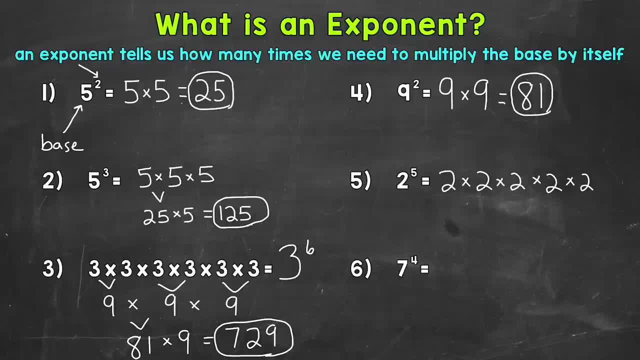 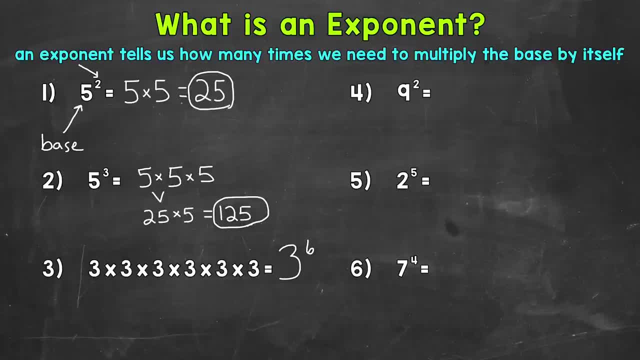 Let's see what this equals. Let's multiply everything here, And there are multiple ways we can think through this And see what this equals. I'm going to pair up all of our 3's here, So we have 3 times 3,, 3 times 3, and 3 times 3.. 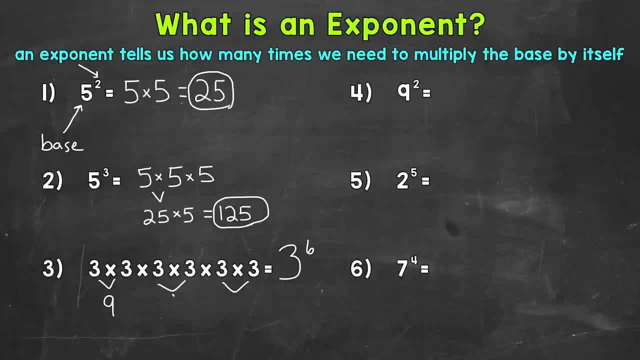 We know that 3 times 3 is 9.. So I'm going to start breaking this down And let's multiply 9 times 9 times 9.. Well, 9 times 9, that's 81.. And 81 times 9, that's going to give us 81.. 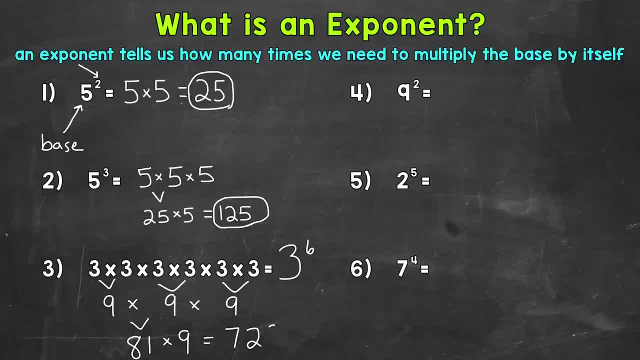 And that's a final answer of 729.. So 3 to the 6th power equals 729.. And, like I mentioned, there are different ways to think through that And different paths you can take in order to get to that 729.. 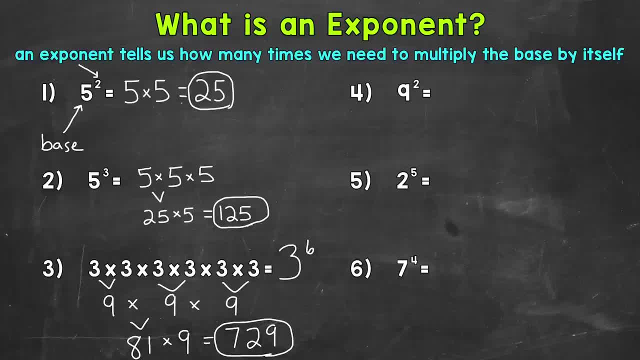 For example, you can just start multiplying 3's as well. So 3 times 3 is 9. Then multiply that 9 by 3. And then that by 3. So on and so forth, Until you use all 6 3's. 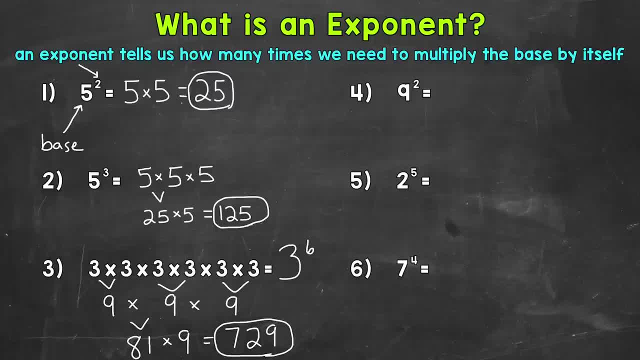 Let's move on to number 4, where we have 9 squared. So this means 9 times 9.. 9 times 9 equals 81. So 9 squared equals 81.. Let's move on to number 5, where we have 2 to the 5th power. 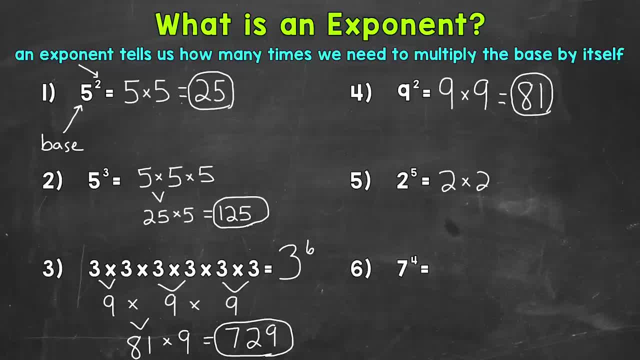 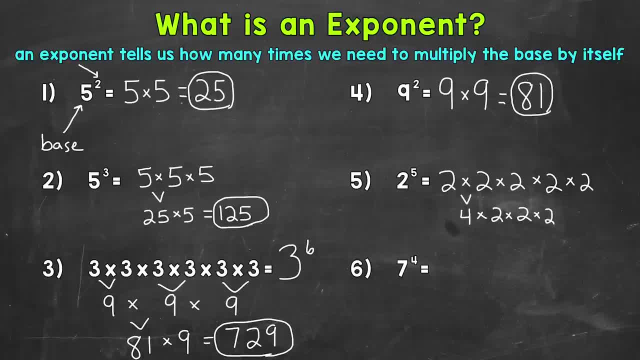 So we have 3 other 2's here. 4 times 2 is 8. And we're left with 2 more 2's. 8 times 2 is 16. And then 1 more 2.. So 16 times 2.. 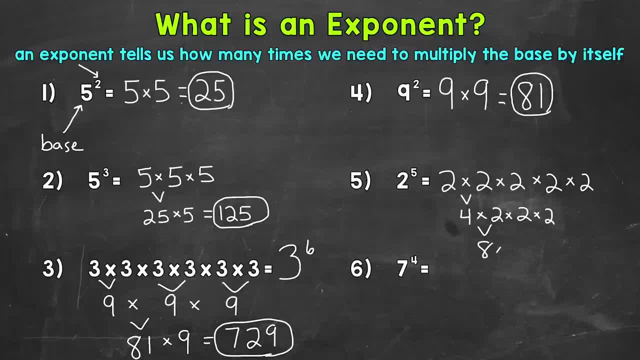 4 times 2 is 8.. And we're left with 2 more 2's. 8 times 2 is 16. And then 1 more 2.. So 16 times 2. That gives us an answer of 32..